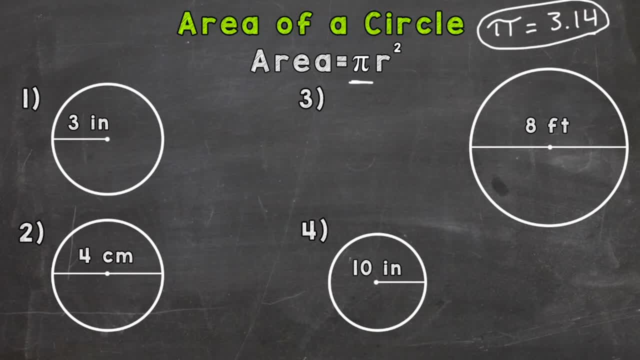 first thing we want to do is write out our formula, So area equals pi times radius squared. Then we want to plug in our radius, So area equals pi times the radius of 3 inches squared. Then we would plug this into a calculator And, like I mentioned earlier, you would hit the pi. 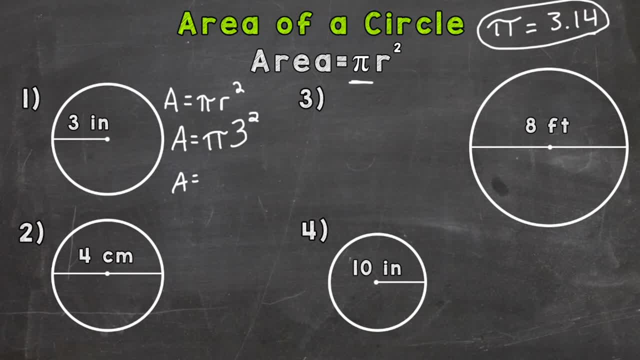 button, Or you can use the rounded, shortened version of 3 and 14 hundredths that is in the top right of your screen. So once that is done, you're going to want to go back to the calculator while you're drawing and remember that the area of 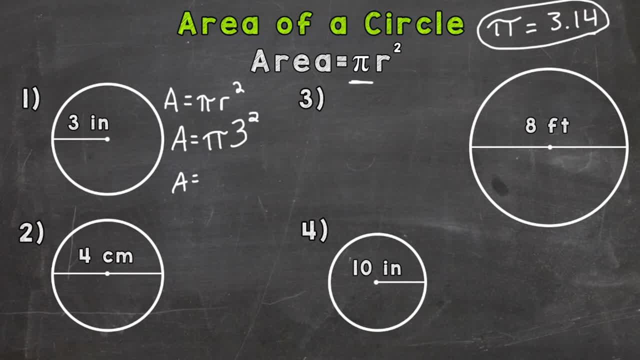 your circle is the same as your radius of 3 and 14 hundredths, And also your radius is the same as your area of 3 and 14 hundredths. So I'm going to round it. So this is a pretty long decimal, so I'm going to round. 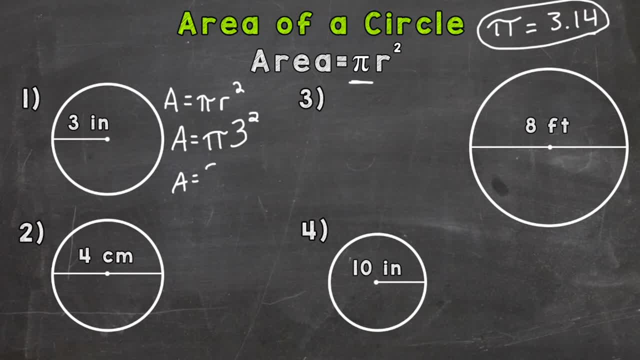 to the hundredths place. So we would have 28 and 27 hundredths square inches And you always square your unit for area because it takes one by one inch squares. it would take 28.27 of them to cover, Or that's five inches. The same thing. if I just did a square, I would have the area of 38.27 of them to cover. 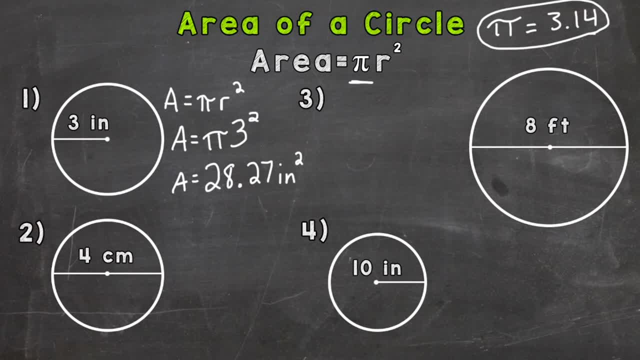 or fill that space for that circle. So if at this point you feel confident enough to try some on your own or at any point during this video, feel free to go ahead of me and then check your answers with mine once I catch up to you. 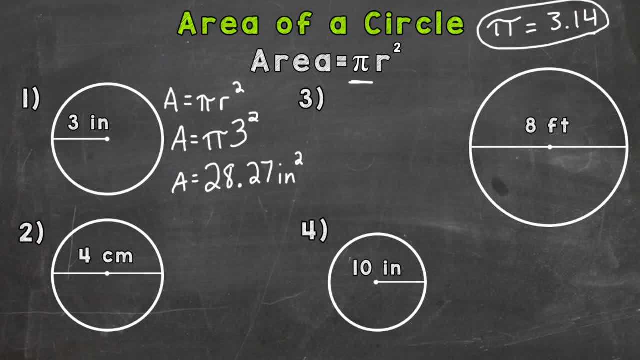 Or if you'd like to work through all four with me, that's fine too. So let's try number two. It's always a good habit to write your formula out first whenever you're using one, whether it's area or a different type of problem. 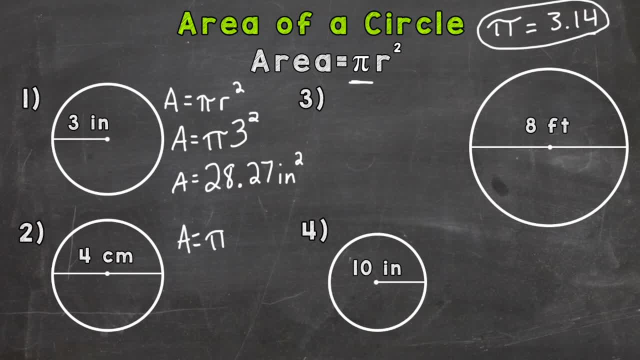 So we have area equals pi times radius squared. So let's plug in. So we have our pi. Now this problem: they give us the diameter. So we only want half the diameter. We want the radius, Which would be 2 centimeters. 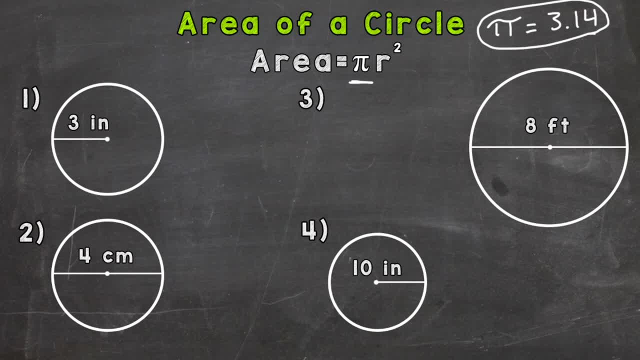 first thing we want to do is write out our formula, So area equals pi times radius squared. Then we want to plug in our radius, So area equals pi times the radius of 3 inches squared. Then we would plug this into a calculator And, like I mentioned earlier, you would hit the pi. 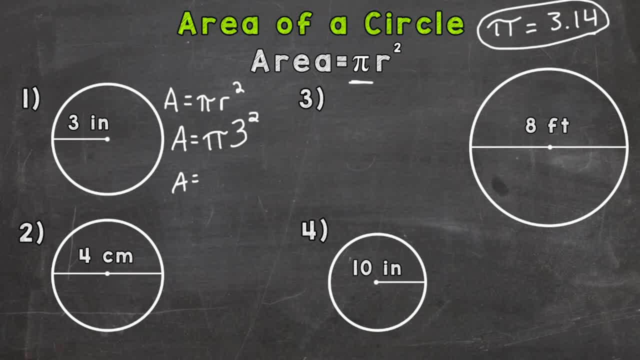 button, Or you can use the rounded, shortened version of 3 and 14 hundredths that is in the top right of your screen. So once that is done, you're going to want to run that down. You want to check out another. 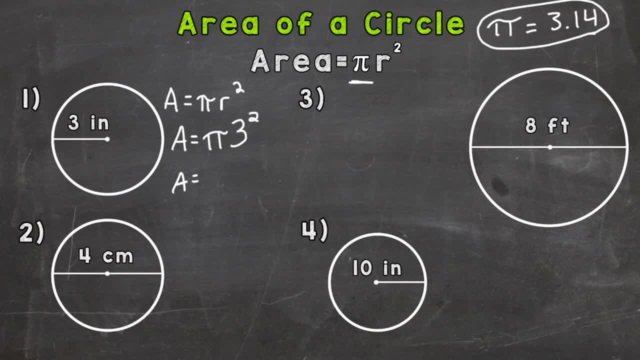 session that I uploaded. we're put back there. here's an into ranking. Alright, so we're gonna do the rounded version of thehandread tweeted and furious version of pi times. Gomez, What we want to do right now is put these together, So you're gonna want to. 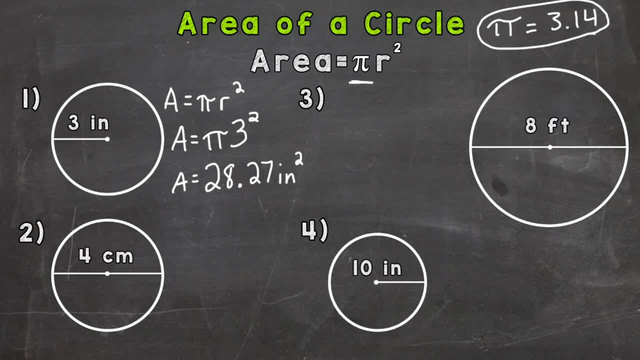 find off the symbol that you have and have bye, bye, And what you're gonna do then is you're gonna need to count our radius. Now, this is an or fill that space for that circle. So if, at this point, you feel confident enough to try some on your own, or if, at any point, 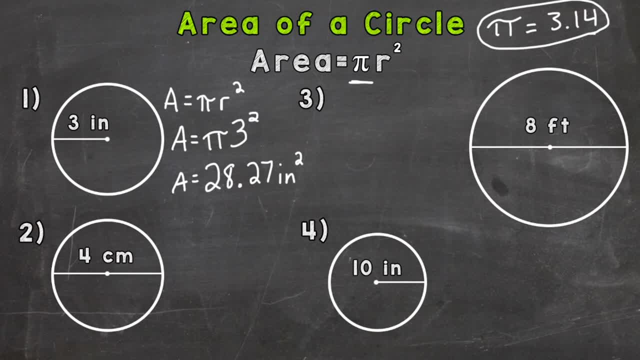 during this video. feel free to go ahead of me and then check your answers with mine once I catch up to you, Or if you'd like to work through all four with me, that's fine too. So let's try number two. It's always a good habit to write your formula out first whenever you're using one, whether 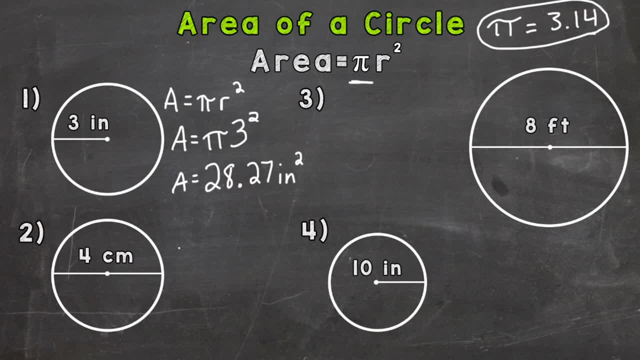 it's area or a different type of problem. So we have area equals pi times radius squared. So let's plug in, So we have our pi. Now this problem: they give us the diameter. So we only want half the diameter, We want the radius. 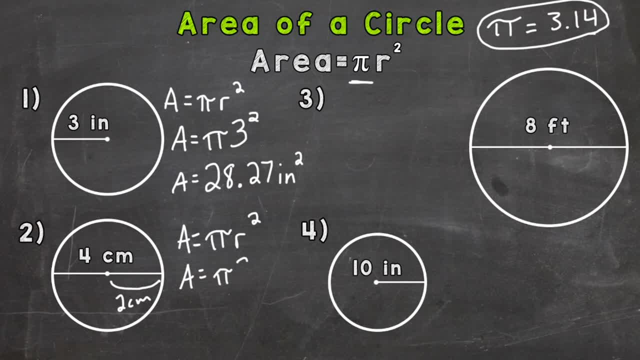 Which would be 2 centimeters. So we plug in 2 for the radius and squared. Once we plug in and calculate, we would get an answer of 12 and 57 hundredths centimeters squared. I forgot to circle my answer for number one, so I'm going to go back and circle that. 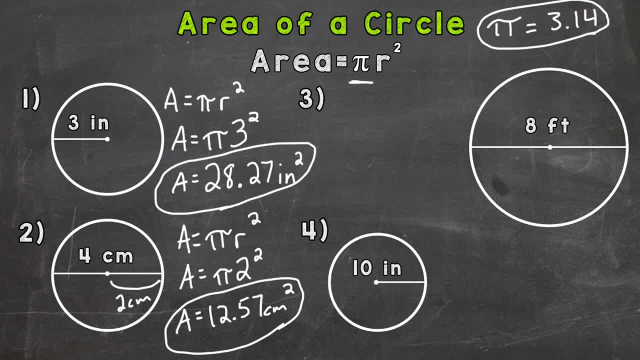 Alright, Let's go to number three. So we start with writing out our formula: Area equals pi times radius squared. So let's put in our Plug in our radius, which would be half the diameter, So 4 feet, So a 4 here. 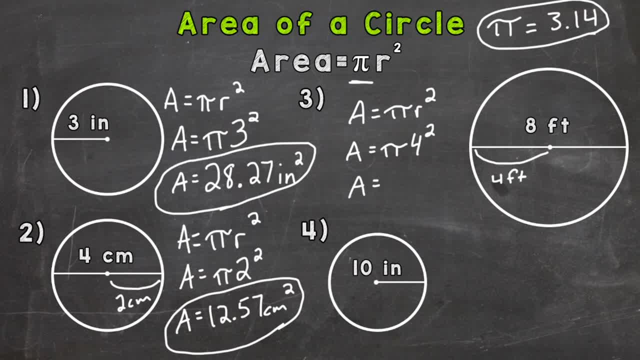 Squared. So once we plug that in, we would get 50.. And 27 hundredths centimeters squared. And again for numbers 2 and 3, just like number 1, our decimal is going to be a fairly long decimal there. so we're rounding to the hundredths place. 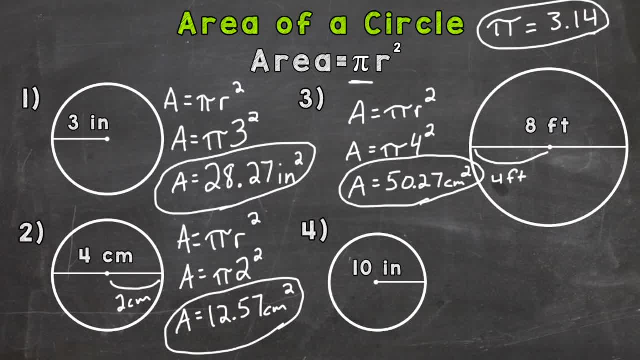 So for number 4, here we are given a radius of 10 inches, so we do not need to take half of that Because, again, that is the radius. You only take half. when you have the diameter. You divide that by 2 in order to get the radius. 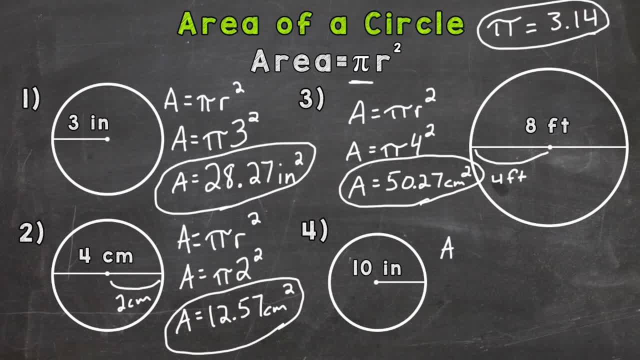 So let's start by writing out our formula: of area equals pi r squared, Then we'll plug in: so our radius of 10 inches, So pi times 10 squared, And we get an answer of 314 and 16 hundredths. 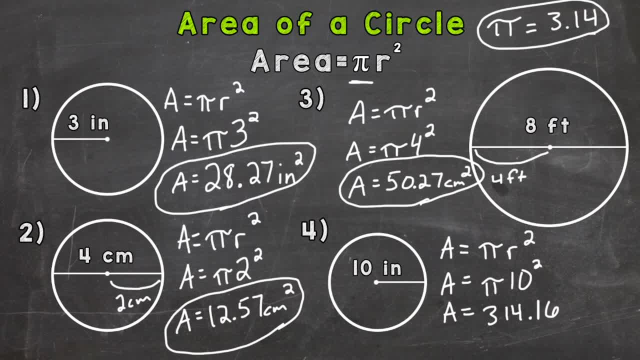 Now again, that's rounded to the hundredths place, because we got a fairly long decimal there. So we round it to the hundredths And our unit is inches And whenever we do area, remember it's square units. So 314 and 16 hundredths square inches. 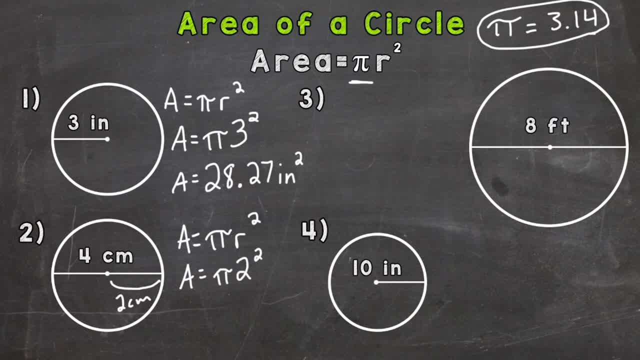 So we plug in 2 for the radius and squared. Once we plug in and calculate, we would get an answer of 12 and 57 hundredths centimeters squared. I forgot to circle my answer for number one, so I'm going to go back and circle that. 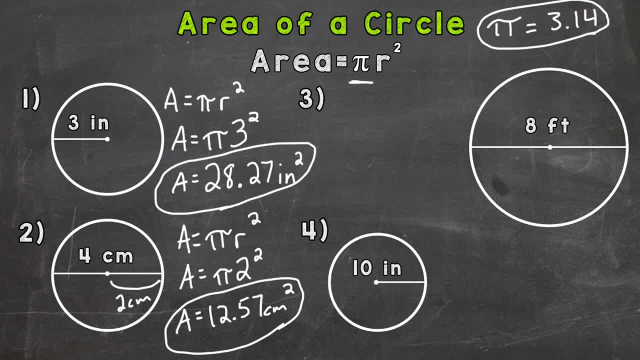 Alright, Let's go to number three. So we start with writing out our formula: Area equals pi times radius squared. So let's plug in our radius, which would be half the diameter, So 4 feet, So a 4 here. 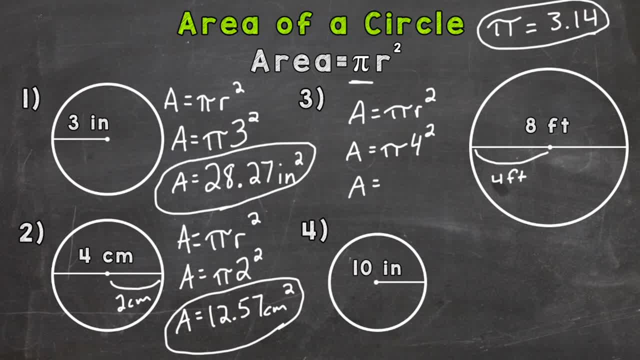 Squared. So once we plug that in, We would get 50.. And 27 hundredths centimeters squared. And again for numbers 2 and 3, just like number 1, our decimal is going to be a fairly long decimal there. 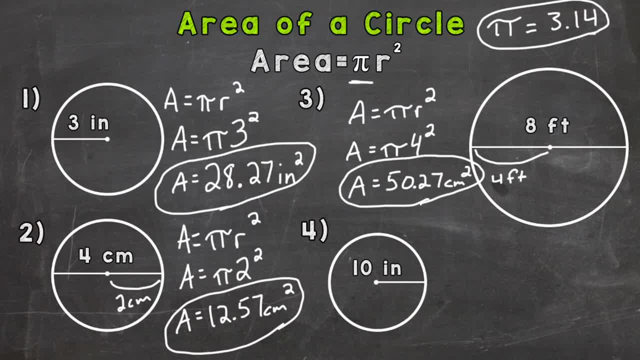 So we're rounding to the hundredths place. So for number 4, here we are given a radius of 10 inches, so we do not need to take half of that Because, again, that is the radius. You only take half when you have the diameter. 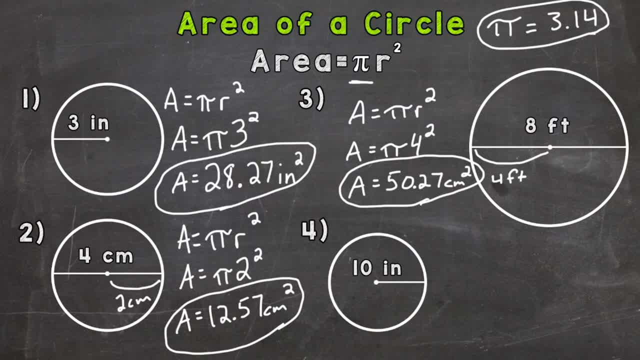 You divide that by 2 in order to get the radius. So let's start by writing out our formula of area equals pi r squared, Then we'll plug in So our radius of 10 inches, So pi times 10 squared, And we get an answer of: 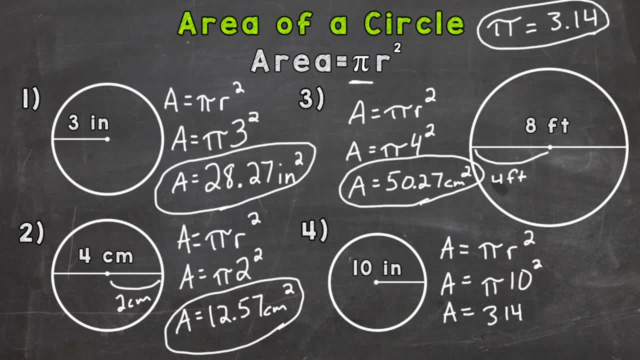 of 314 and 16 hundredths. Now, again, that's rounded to the hundredths place, because we got a fairly long decimal there. So we rounded to the hundredths and our unit is inches And whenever we do area, remember it's square units. So 314 and 16 hundredths square inches. So there you have it. 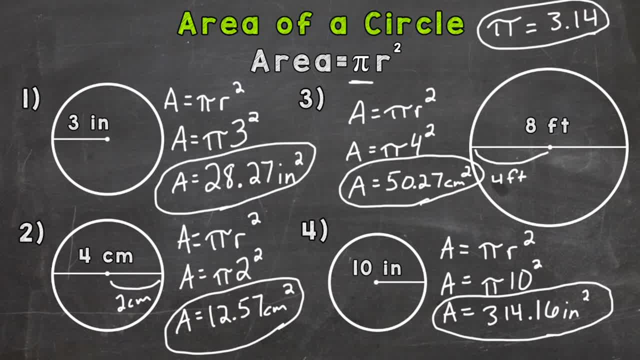 There's how you calculate the area of a circle. Hopefully that was helpful. Thanks so much for watching, Until next time, peace.